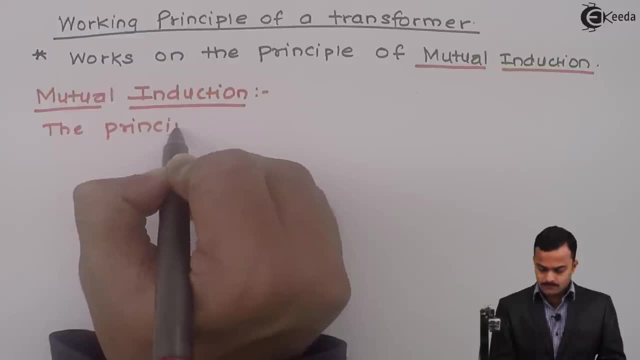 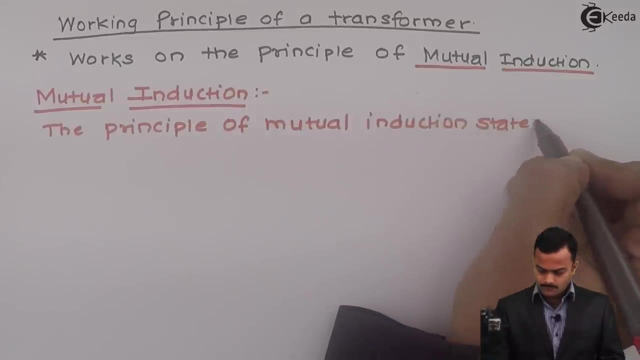 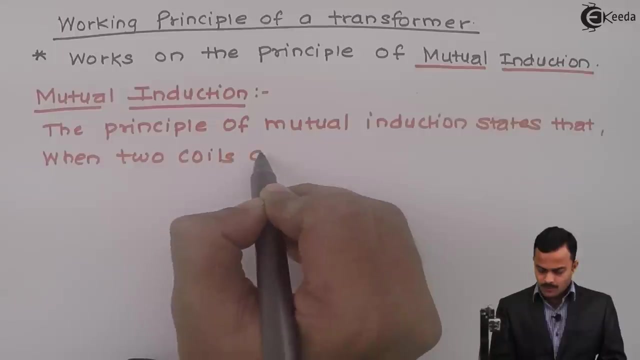 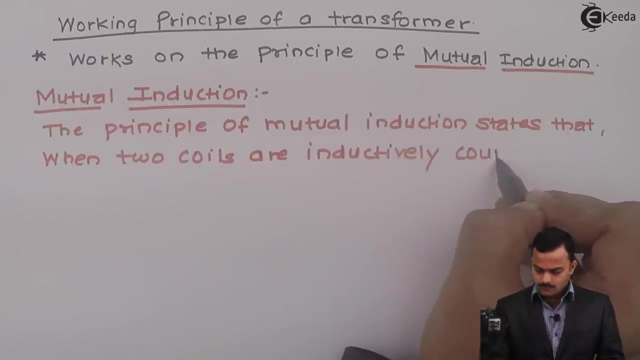 The principle of mutual induction states that the principle of mutual induction states that when two coils are inductively coupled, and if current in one coil is equal to the current in the other coil, and if current in one coil is equal to the current in the other coil, 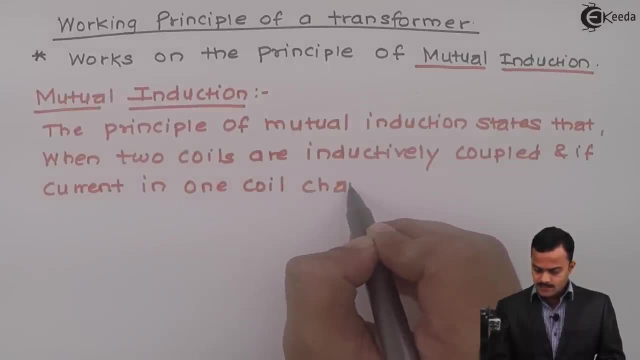 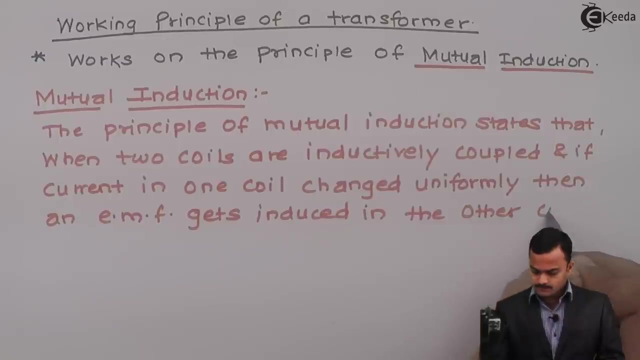 and if current in one coil is equal to the current in the other coil, changed uniformly, then an EMF gets induced in the other coil. So what it's saying, Suppose I am placing two coils together without having any electrical connections between them. that is what it is called as. 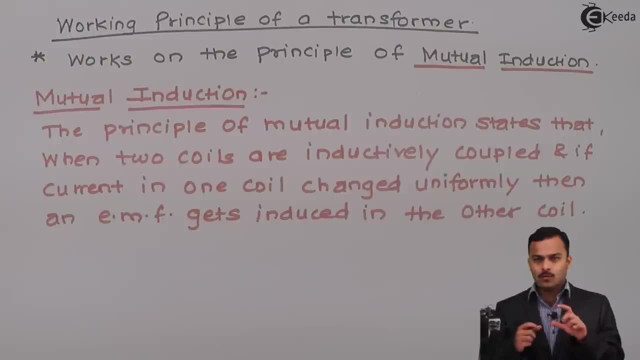 inductively coupled and i'm exciting, one of the coil by giving ac supply. so what will happen? emf will get induced at the secondary side. this concept is called as mutual induction. so what happened basically? that i will explain with the help of basic transformer diagram. 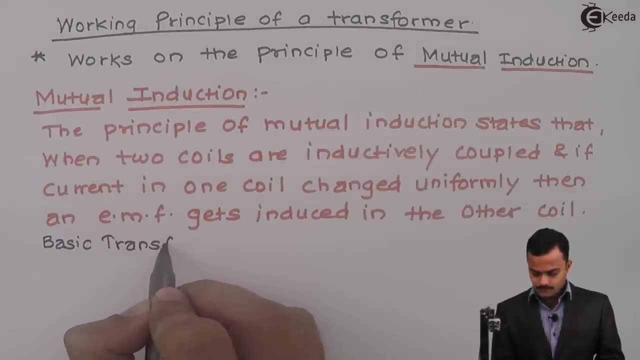 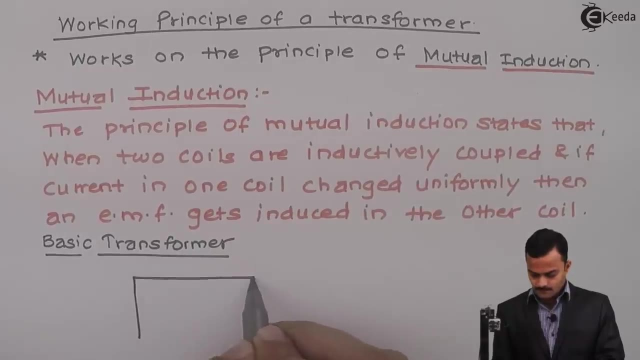 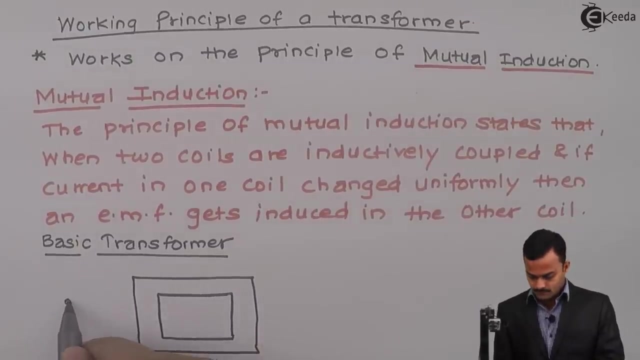 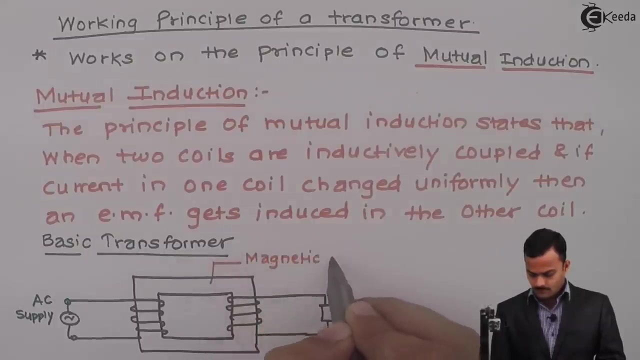 it is like this. so in this structure, this is the magnetic core. on this core, two coils are wound like this: this coil we call as a primary winding, so so this coil is called as a secondary winding and this winding, or this coil, is called as secondary winding. 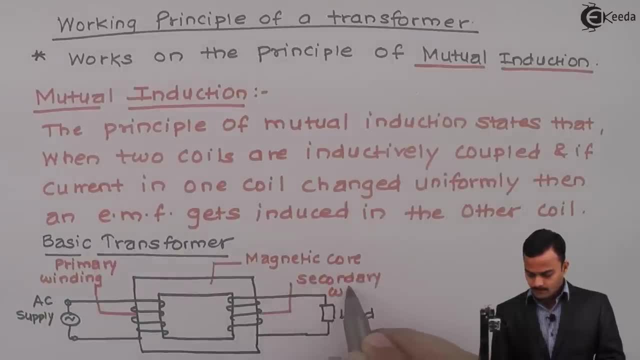 now how to decide primary and secondary winding. wherever there is a supply connected, that coil is called as a primary winding, and wherever load is connected, that coil is a secondary winding. now, because of this, ac supply current will pass through this. this current will give rise to magnetic flux, which will 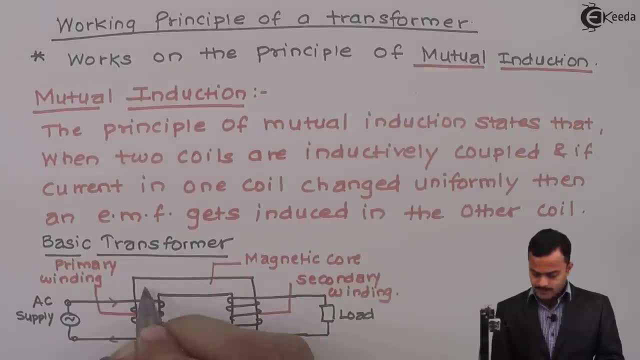 pass through this magnetic core like this. so this is magnetic flux. fine, now what happened? this magnetic flux, which is changing with respect to time, gets linked with a primary winding and will give rise to a emf by faraday's law of electromagnetic induction, and that emf is called as self-induced emf. what is? 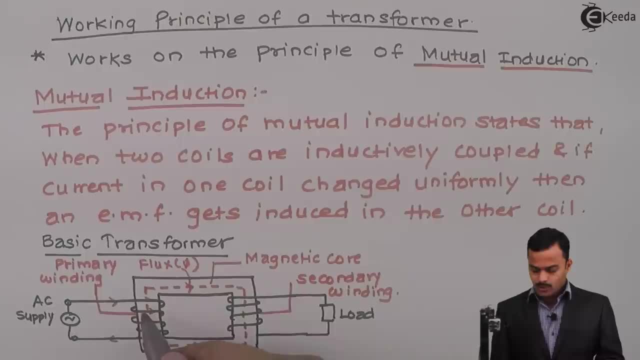 the self-induction. i am getting a voltage because of a sub-magnetic flux. so this is magnetic flux. so this is magnetic flux. so this is magnetic flux which is connected to same coil, but at the secondary side, what will happen? same flux is linked with a secondary winding also. so this flux which is changing with respect, 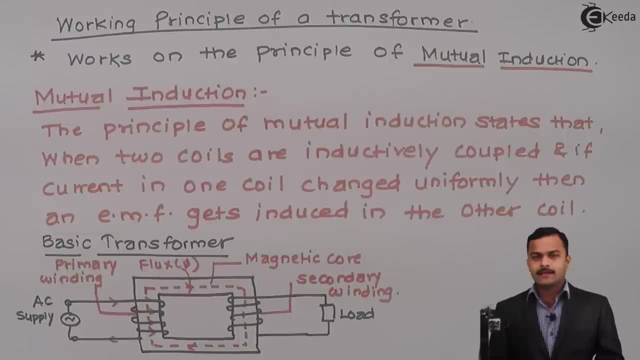 to time gets linked with a secondary coil, give rise to a emf. this emf got induced because of the supply which is there at the primary side. therefore it is called as a mutually induced emf And if I connect the secondary winding through, load current will pass through the secondary side also. 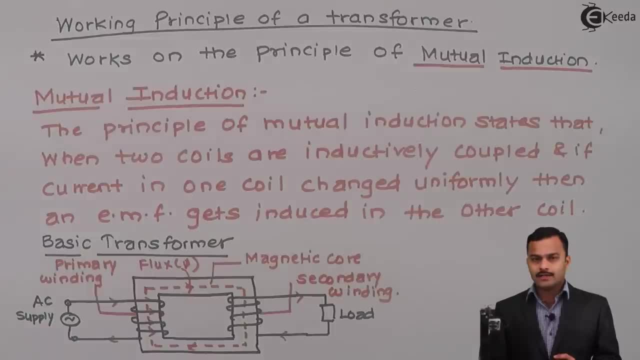 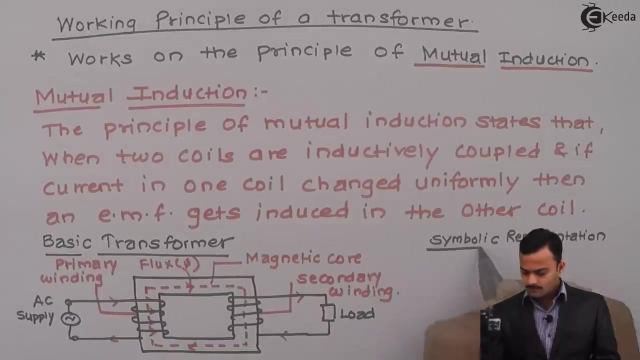 So this is what the principle of mutual induction. So I have explained that concept with the help of a basic transformer. Now how this basic transformer can be represented. So I am going for symbolic representation. So it is very simple.